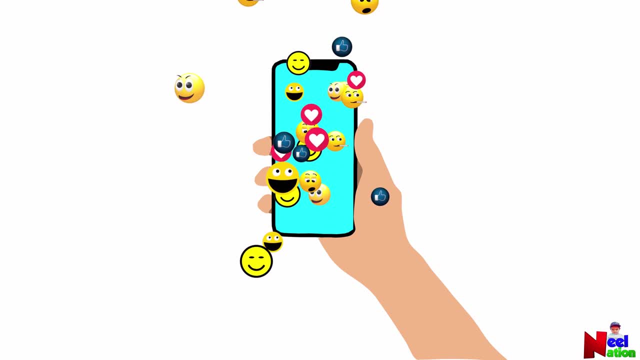 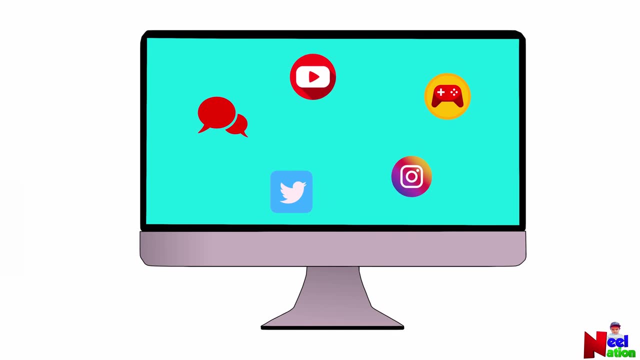 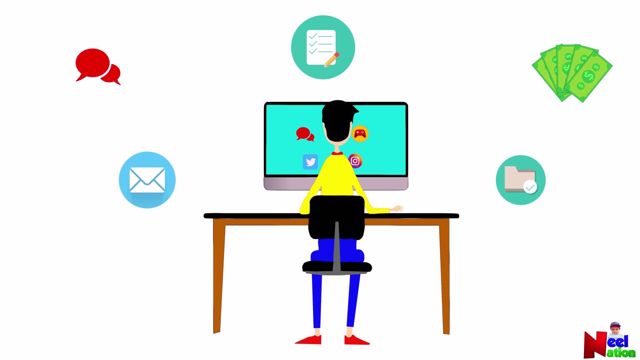 to the internet. A phone connected to the internet is like the world at your fingertips. The internet can be a fun place, but at the same time, it can be a dangerous place to be in if you are not careful. Internet thieves, who are also known as cyber criminals, 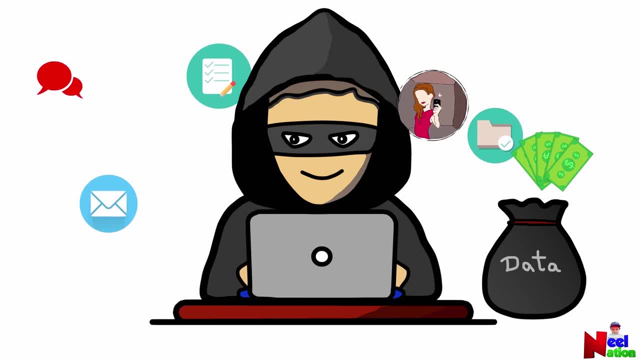 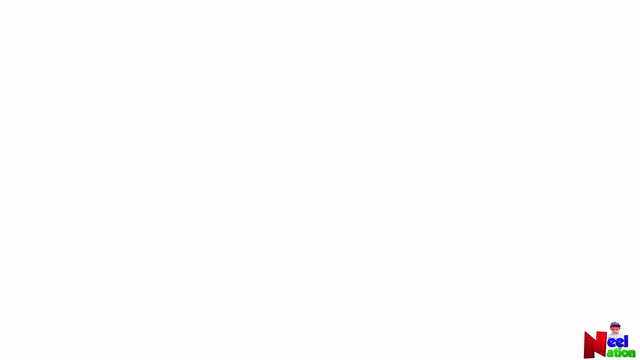 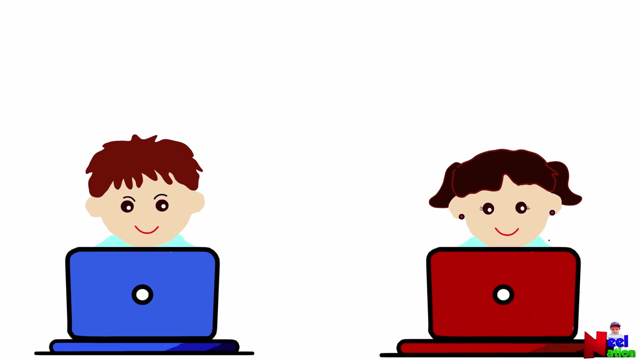 can break into your computer and steal your personal data. Now let's learn about staying safe on the internet. Tip number one: Do not open emails from strangers. Email is a message that is sent and received using computers. It is an important form of 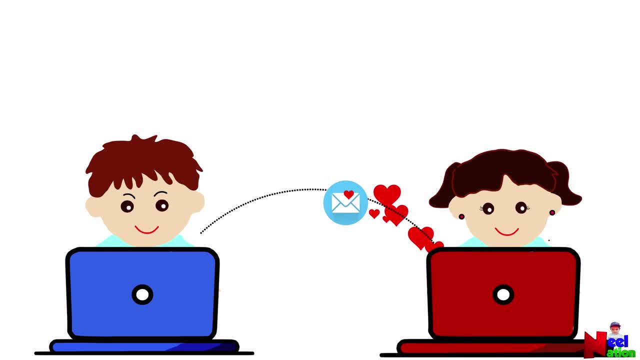 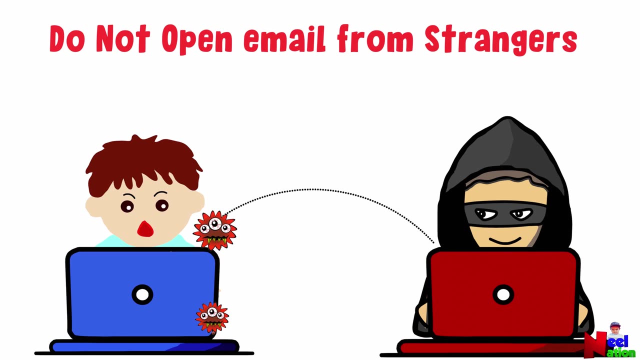 fast communication that allows people to contact one another and share information all over the world. But you must be very careful when you open an email from strangers. Some emails can contain computer viruses that can infect your computer and wipe the entire data from your computer. always check with an adult before opening emails from strangers. tip number two: you never share your. 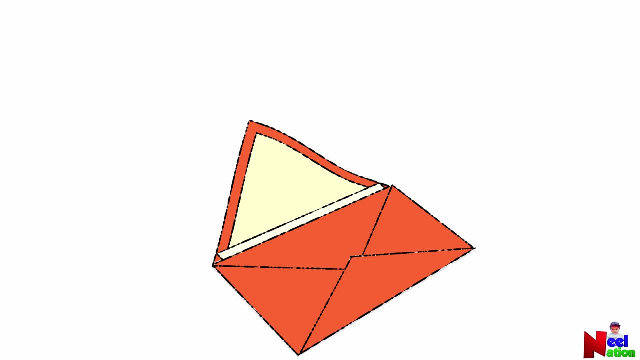 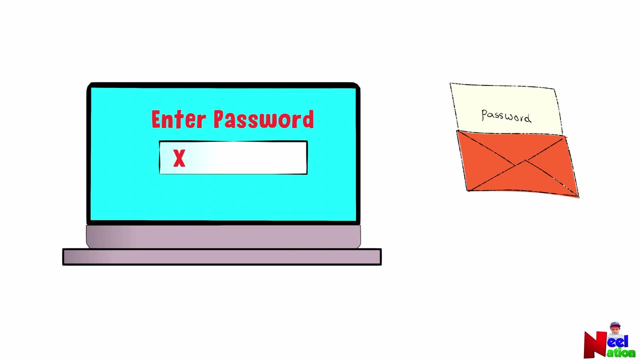 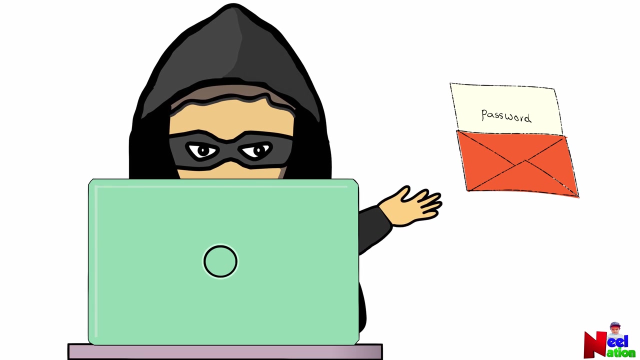 password with others. password is a secret word or phrase that a person must know to be allowed to enter a computer system. you should always try to use longer password. password must always be a secret in the digital world. the bad guys are called cyber criminals if they can figure out. 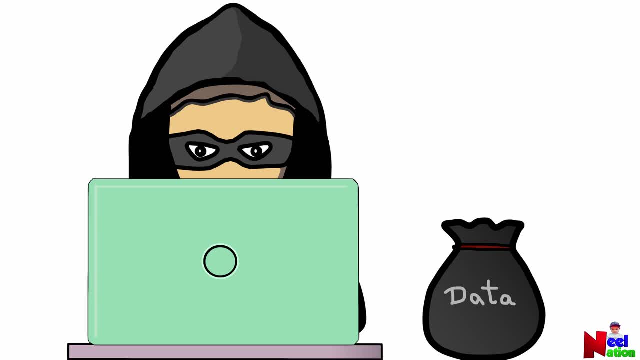 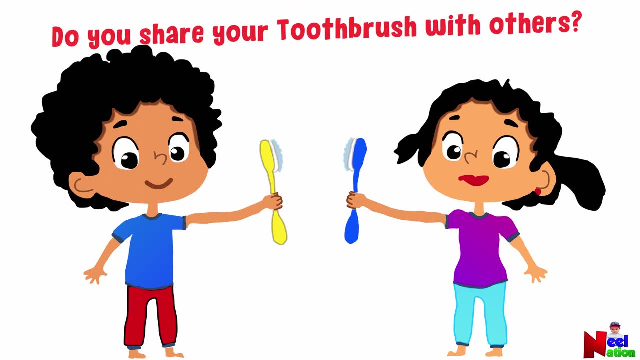 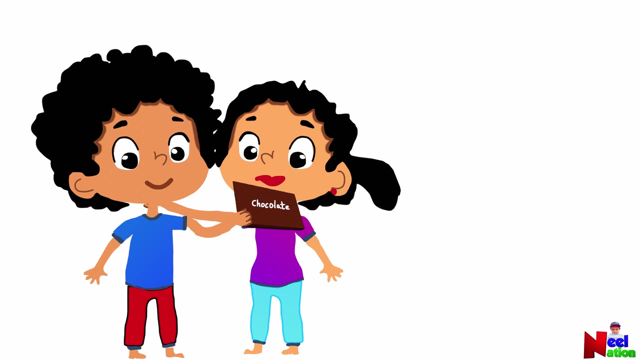 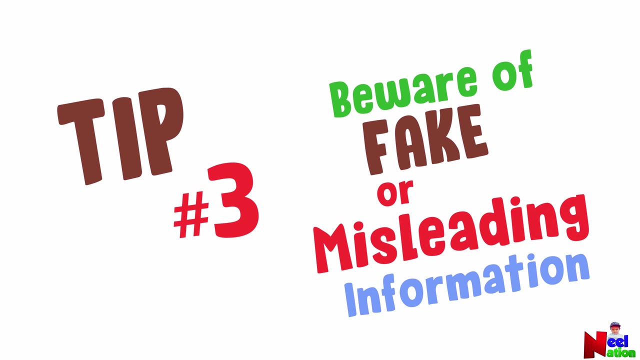 a person's password. they can access their private information using that password. now let me ask you something. do you share your toothbrush with others? no, correct passwords are like your toothbrush: you never share your password with others. you can share chocolate, but not your password. tip number three: beware of fake or misleading information. please be aware that the things that